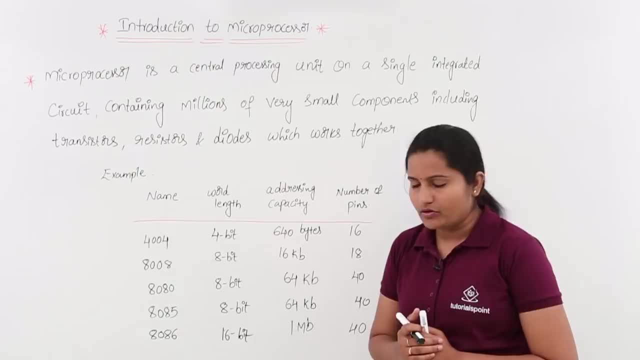 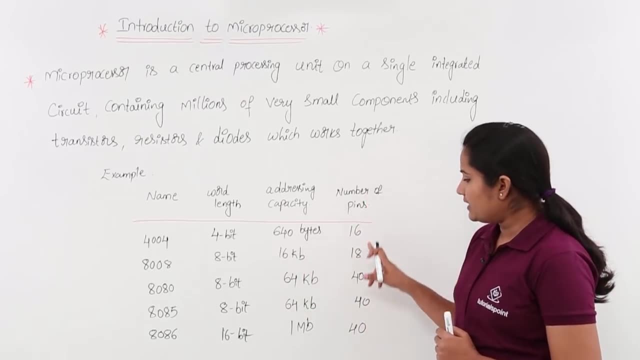 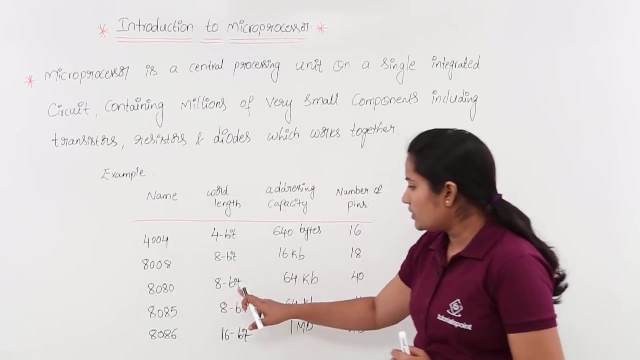 increasing from one micro processor to another micro processor. So this is 16 KB addressing capacity. this is having 16 KB addressing capacity and the number of pins are 18.. So like that we are having next micro processor 8080.. So here, 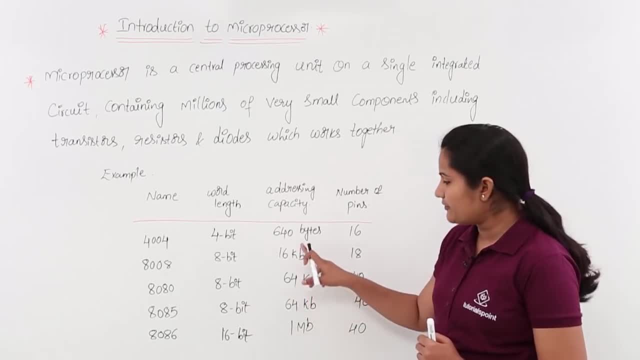 also, the world ends is 8 bit, but addressing capacity is increased from 16 KB to 64 pin. So if gekommen to 6 bit, end okay. So using child's brain we can say primary decrease in pin number storage. Similarly Tитian in this T Lt. frankly we can say: 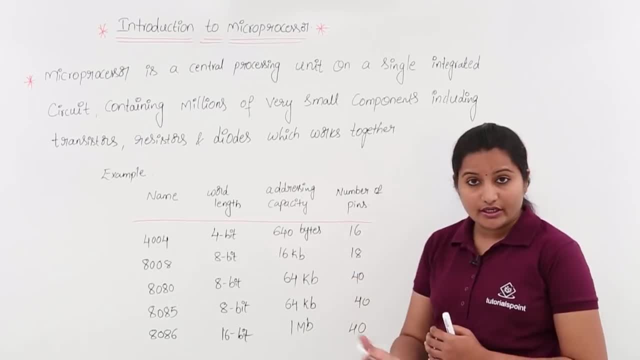 how many pin values you have in T Lt. So basically their first example, or Now 5 products. if familiar with T La elementary unit, there are many postا, but in computer, for example, 64 KB. Now the number of pins also increased. in this microprocessor the number of pins are 40. 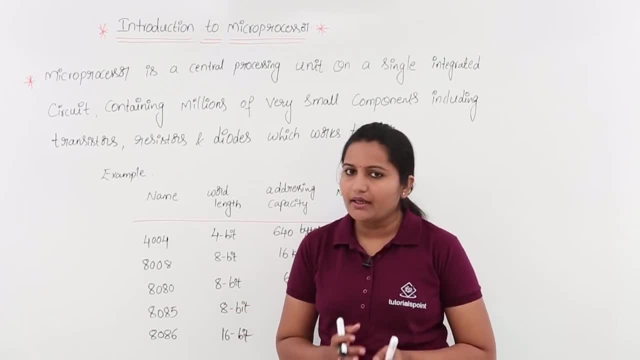 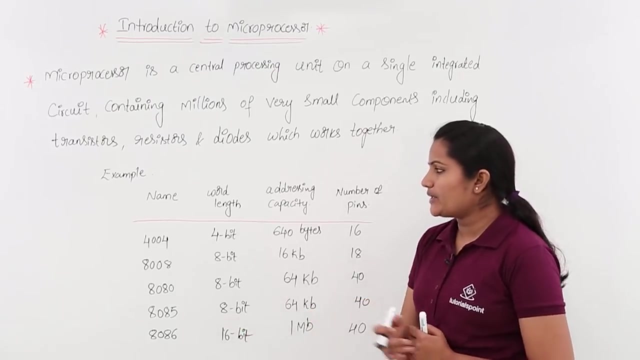 here And coming to 8085, this is very important microprocessor that we need to discuss because in any technical exams they will ask 8085 and 8086 only. So here for 8085 microprocessor. this is also 8 bit volt length. that means 8 bit microprocessor, and here it is having 64 KB. 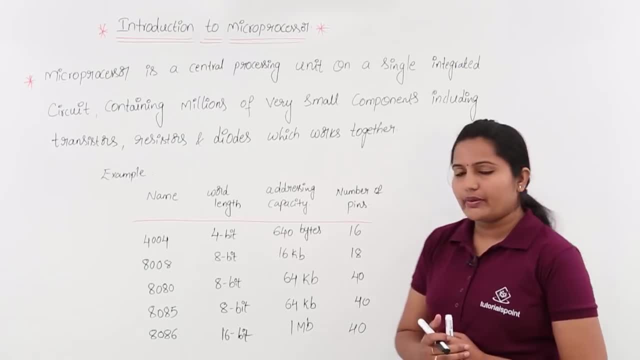 addressing capacity And coming to the number of pins, from here onwards you are having 40 pin ICs. that means for 8085 IC we are having 40 pins. So here we are having 8086 microprocessor, in which 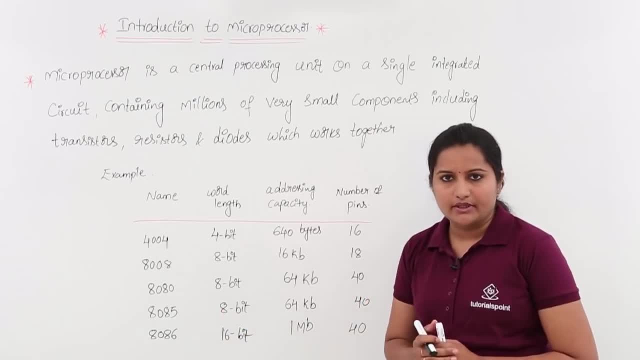 the volt length is increased from 8 bits to 16 bits. From this onwards, our microprocessor is also increasing from 8 bits to 16 bits. So here we are having 8086 microprocessor in which the volt length is increased from 8 bits to 16 bits From this onwards. 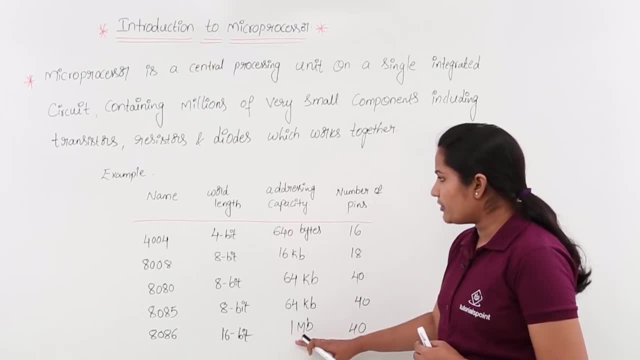 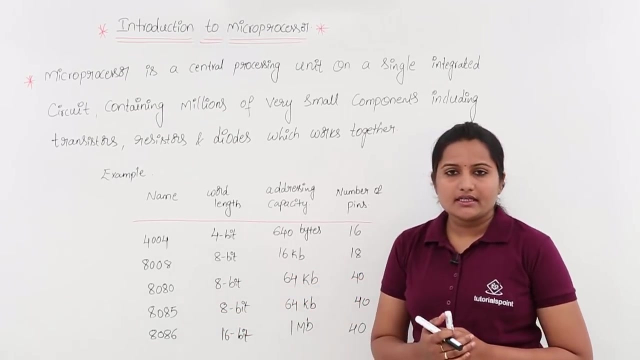 our microprocessor is also increasing from 8 bits to 16 bits, So for this the addressing capacity is 1 MB, and here the pins are same, with same 40 pins. here volt length is increased and addressing capacity is increased. So 8085 and 8086 are very important for any technical point. 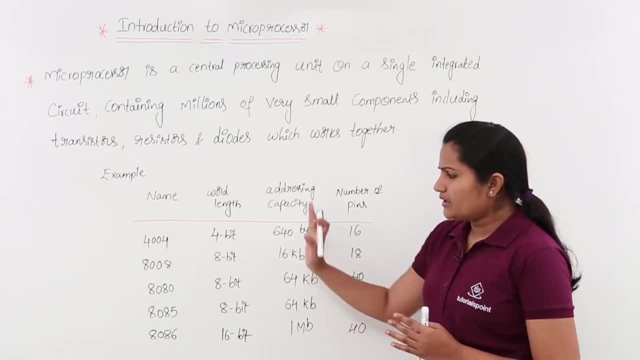 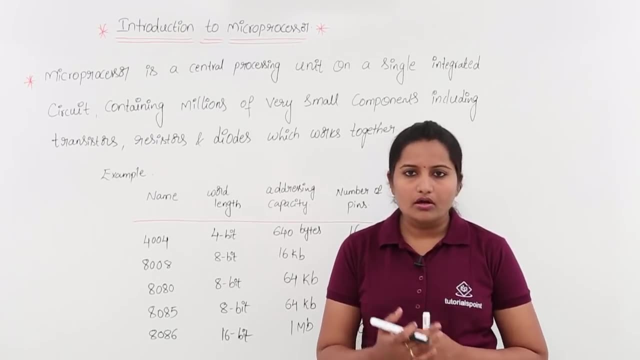 of view, technical exam point of view Here, not only this microprocessor. we are having so many microprocessors like Pentium and Pentium, Pentium 2, all these we are having as our microprocessors, which we are using widely in.